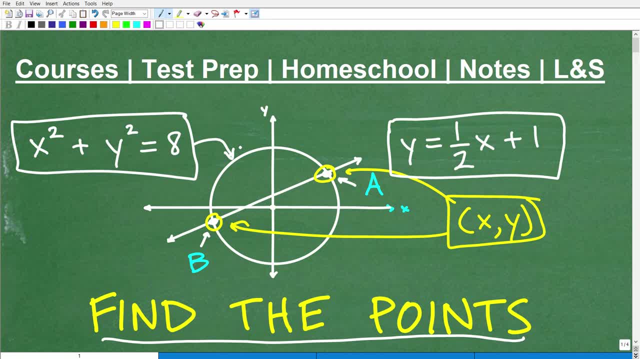 mathematics, Even if you're at a more basic level. it might be challenging for you. But you know, just because something is challenging doesn't mean that you can. you know you're not going to be successful, right, What you need is great math instruction. 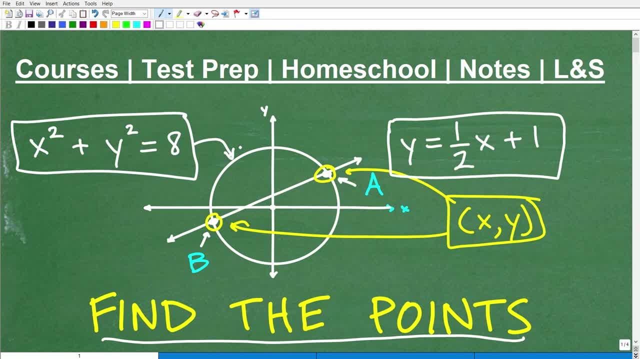 math instruction that is understandable and comprehensive and makes sense to you. Okay, And that's what I like to try to do, not only in my videos, but in my full math program. So if you need help in your current math course or maybe some sort of special test that you're- 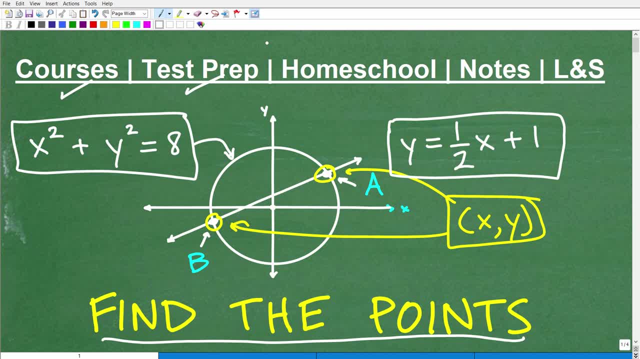 getting ready for that has math. I'm talking about things like the SAT, ACT, teacher certification exam, GED or, if you're homeschooling mathematics, check out my math to help program. I'm going to leave a link to it in the description of this video. I literally have over a hundred plus. 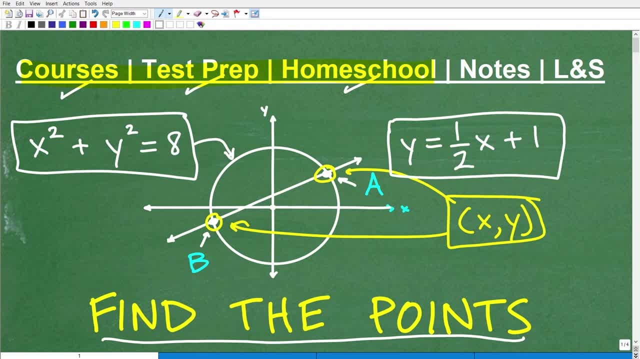 different math courses that span all these categories and much, much more. I'm also going to leave links to my math notes in the description as well, because so many students do not take adequate math notes. They kind of take notes, you know, on some days they're like yeah. 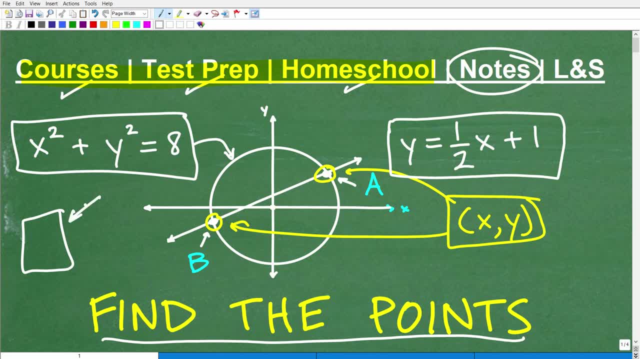 I'll take notes. other days They don't take notes. but here's the deal: If you can, if your notes aren't, aren't uh of the quality where you can give your notes to someone else and they can look at it and say: well, you know, I'm not good at math, I'm not good at math, I'm not. 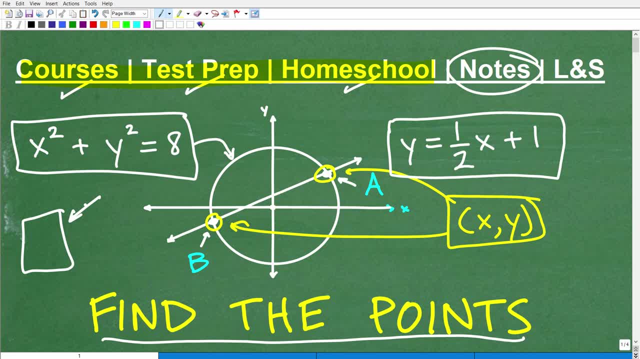 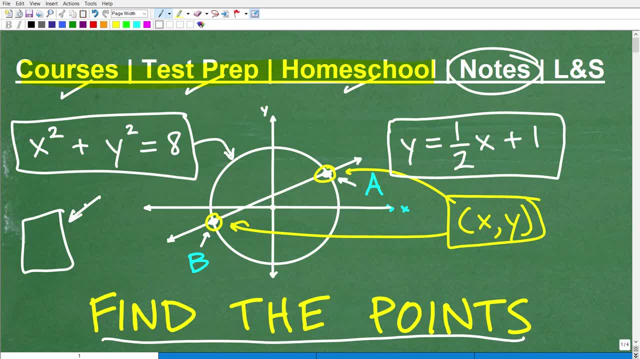 a lot of focus and work, but if you're focused and work in your math class, you're going to be learning more. So take better notes and everything will get much better. But in the meantime, you can use my notes if you like, And if this video helps you out, don't forget to like and subscribe as. 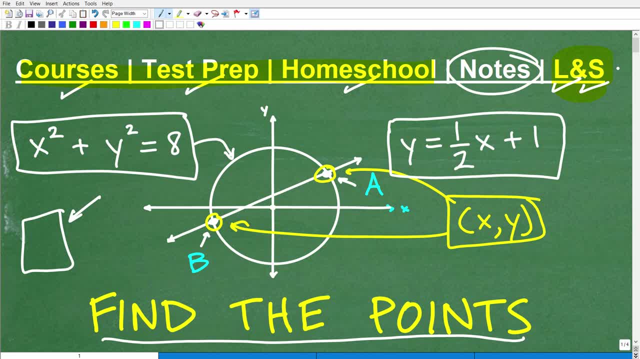 that definitely helps me out. Okay, So let's go ahead and show you the answer here. So we're looking for the location of point a and point B and I'm going to give you those coordinates in terms of X, Y, point. 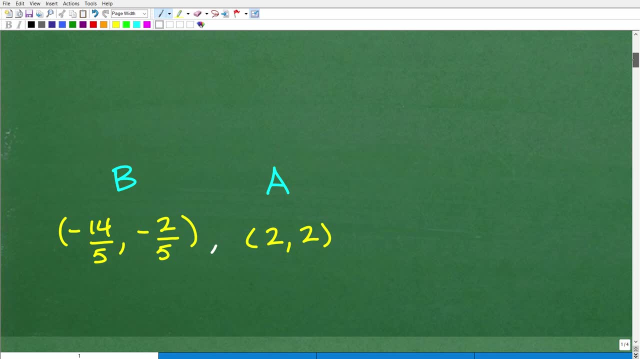 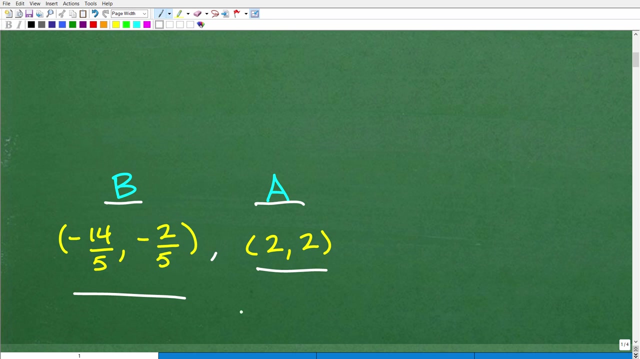 So let's go ahead and take a look at the answer right now. Okay, So point a is that the coordinate two, two, and point B of the intersection between that circle and line is that negative 14 or five comma, negative two fifths. So those are the two points, Okay. So how did you do Well? 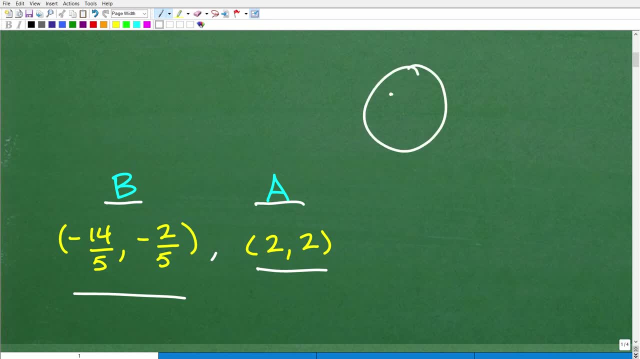 if you got this right, that's pretty impressive. Matter of fact, I'm going to give you a nice little happy face and a plus, and I'm going to actually give you more than a hundred percent. I'm going to give you like 120%. back in my days in the 1970s and eighties- the most you could get. 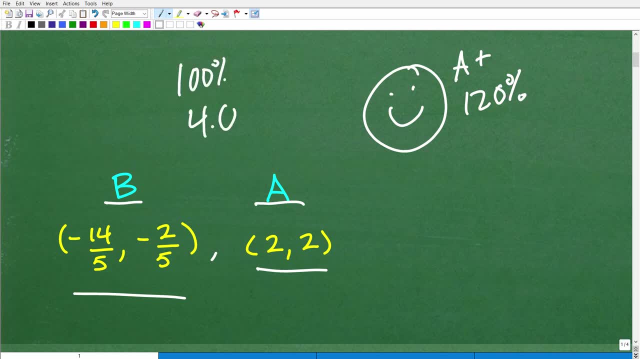 was typically a hundred percent And your GPA, if you were like perfect, was 4.0, but nowadays you can get like 180%. You can get GPAs of like 9.2.. It's pretty crazy, But anyways, listen, I'm going to. 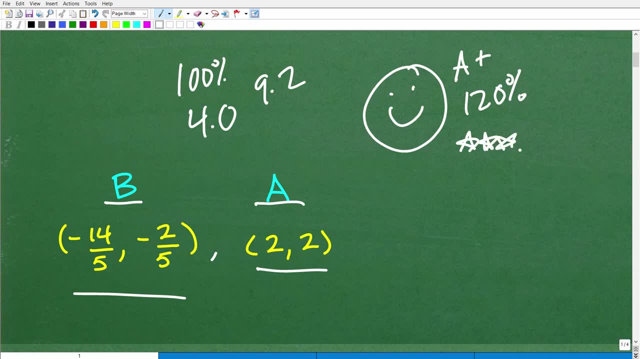 give you that eight plus a hundred percent and multiple stars to celebrate your awesomeness with algebra word prompts. Very, very good. Now if you were looking at this problem and you're like: ah, I think I was doing it right. you know what do I? 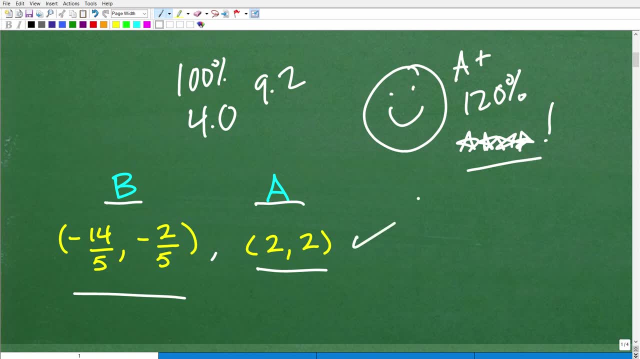 need to do. Well, let's go ahead and get to get into this right now, because, even though you may not have gotten the correct solution, you very well could have been on the right path. So that's why I encourage all of you to attempt these problems. write things down, because, again, 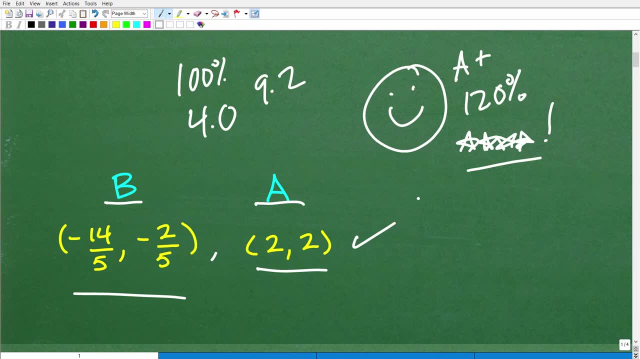 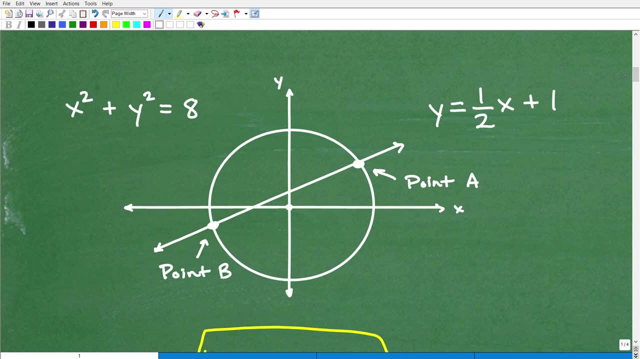 you very well could have been on the right path, but maybe you ran into a stumbling block. but let's go ahead and take a look at what's going on here And really what we're dealing with is what we're dealing with is a system of non-linear equations. Let me back up here real quick. 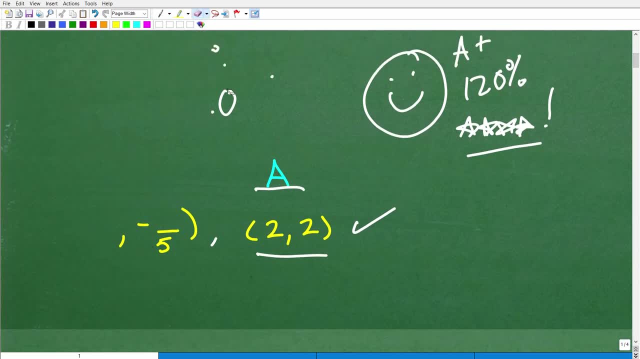 and let's just erase all of this so I could just show you here real quick. Now this is a topic that I'm going to be talking about here. It's something that all of you should have learned back in Algebra 1 or pre-algebra. So let's just draw a little xy coordinate plane here. 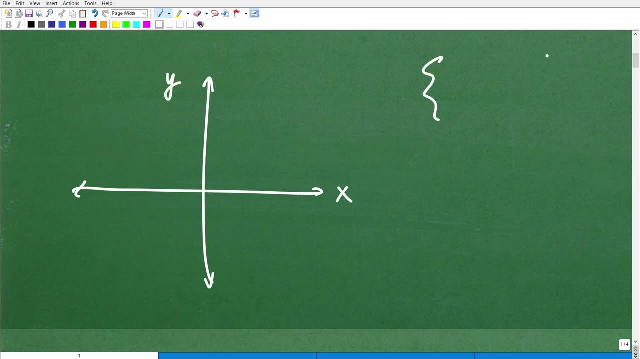 So here's x and here's y. So here let's say we have a system: y equals 2x plus 1, and let's say 2x minus y is equal to 7.. Now I'm not going to think about this too much and actually give you the. 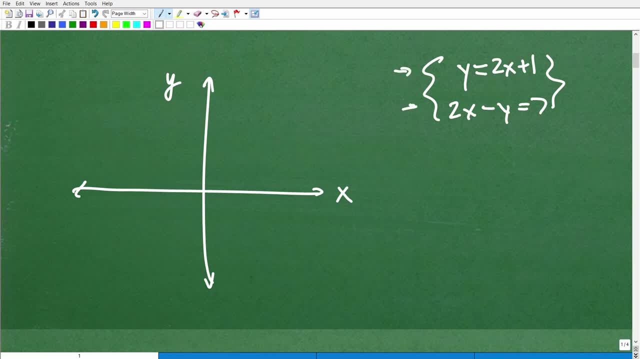 exact graphs to both of these, but this is a line and this is another line. Okay, so let's suppose I graph one line here and I graph another line right here. That's a terrible line. I could do better than that. Let's use a different color, by the way. Let's 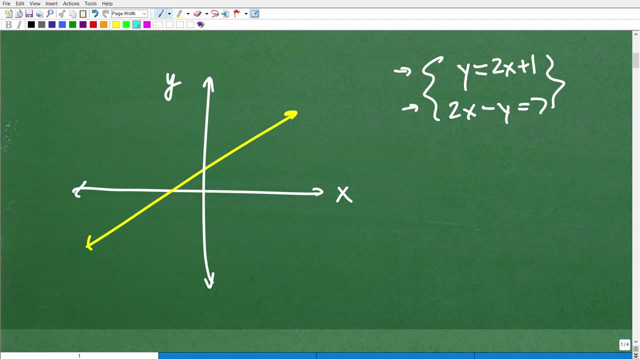 hold on one second. I'm trying to get it together. All right, let's see There you go. I'm going to use blue, All right, so here is another line. I'm going to use blue, All right, so here is another. 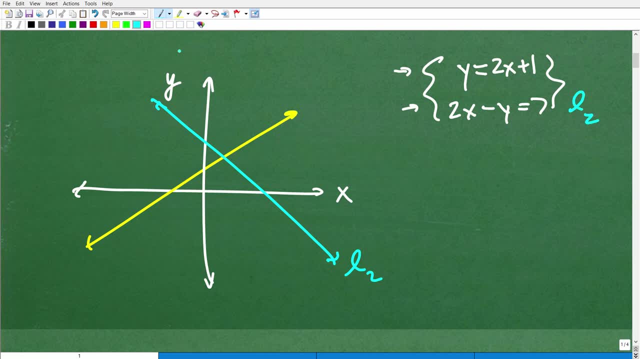 line. So this would be, let's say, line 2.. This would be line 2 and this would be line 1.. Line 1.. Okay, so again we're talking about stuff that you learn, as even in pre-algebra you got introduced. 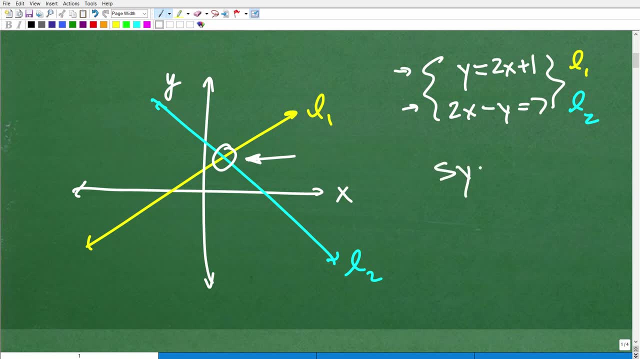 to basic systems, All right. so the topic we're dealing with here is systems. All right, but we're dealing with what we call two variable linear systems. Okay, two variable linear systems, And effectively what we're doing is conceptually, 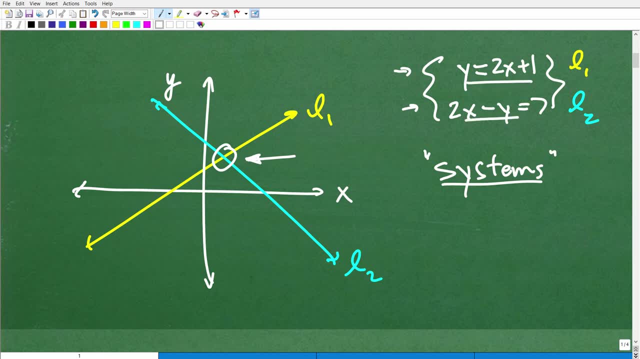 is that these systems represent lines. These are linear systems, so it's one line, another line, And if these two lines happen to cross this point of intersection, this xy point here would be the solution to the system. Okay, now, of course, the lines don't have to cross, and 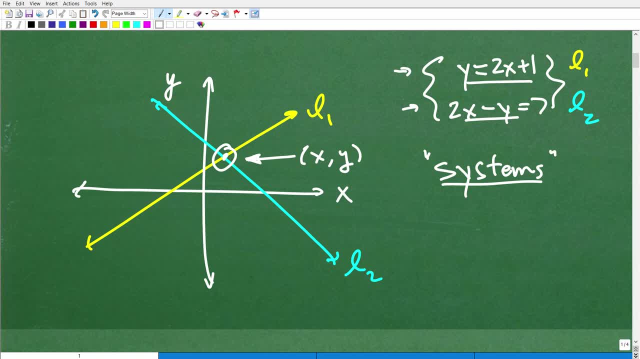 the lines can be parallel where there is no solution. But anyways, hopefully you get the general idea. But what we're talking about here again is linear systems, ie systems that involve a line. But what we're talking about here again is linear systems, ie systems that involve a line. 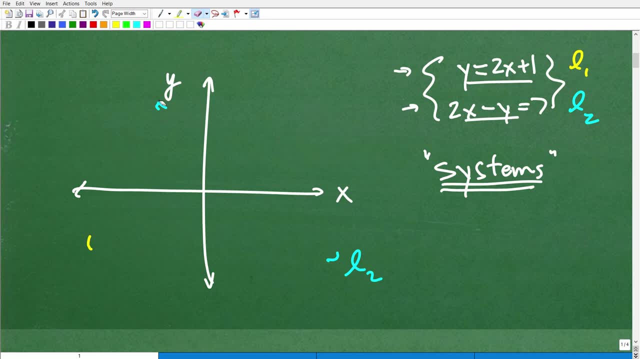 But what we're talking about here again is linear systems, ie systems that involve a line. But what? But what about systems that involve a circle and a line? OK, so, instead of two lines, right, let's just kind of fix up our little system here. 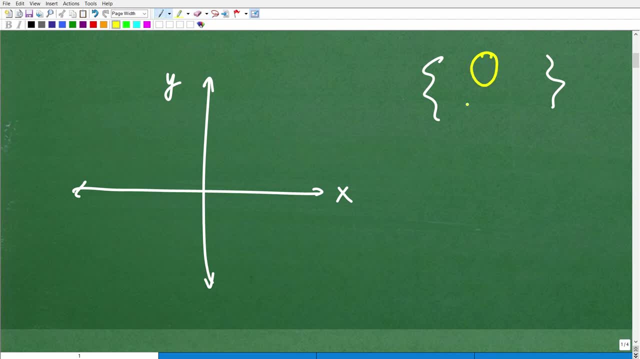 OK, what if we had a circle and a line? OK, well, that's our situation here, So we have a circle and then we have a line. So again, the points of intersection, if these two objects do in fact intersect. 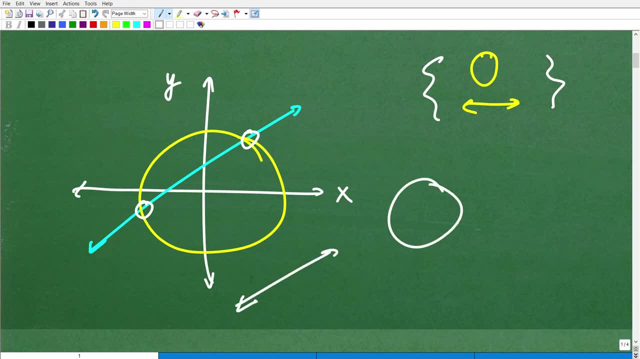 because here's the thing- I could have a circle like this and I can have my line over here where I have no points of intersection. So they may- they may not be a solution to this system, But really the topic, what I'm kind of getting at here, is systems of nonlinear, nonlinear equations. 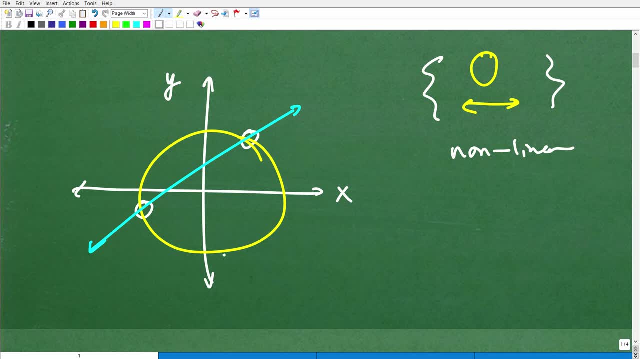 Now, even though we have a line, we do have a circle. OK, so what if I had a circle and I had like an exponential function? Right, Let's kind of fix this thing up. Something like this: Right Again, nonlinear. you're still looking for points of intersection. 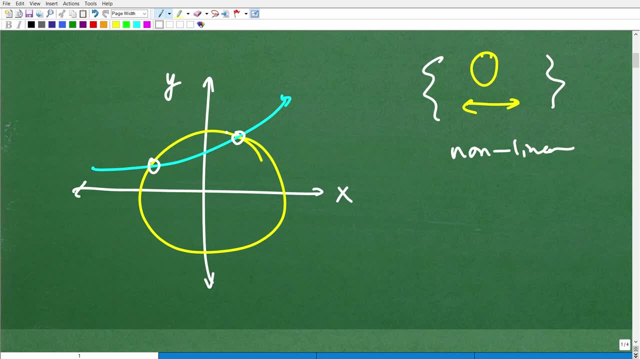 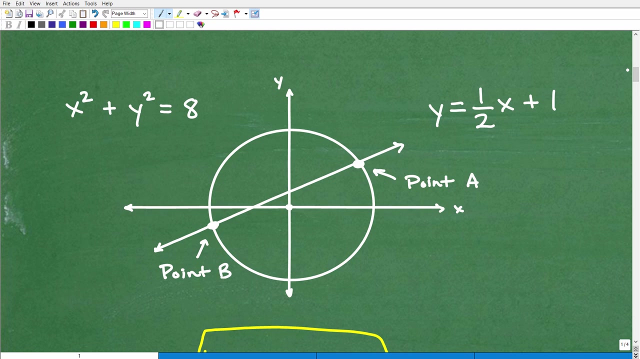 So the skills that you learn to solve linear systems like the substitution method and linear combination method and graphing method, those type of basic techniques you can actually use to solve this problem. So, anyways, hopefully this kind of will set up. you know how to solve this, these type of problems. 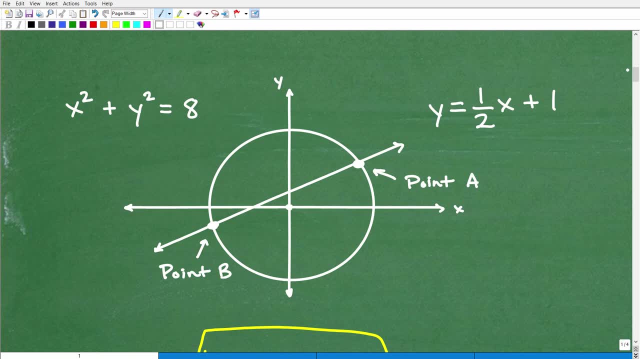 It's not just. you know, in math it's like: here I'm going to show you how to solve this one problem, But if you don't understand the big picture, well, then you're not going to be able to apply this in a more general sense. 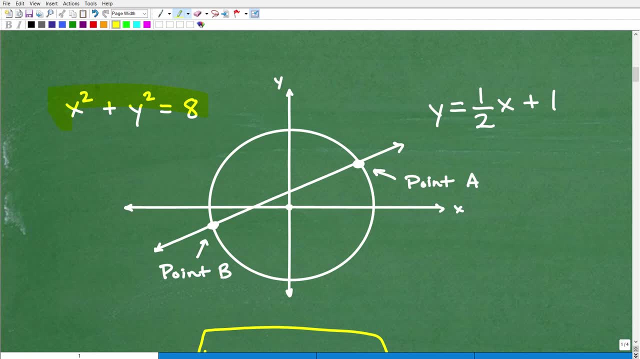 OK, All right, So here is our equation for the circle. Now, I'm not going to get into the equations of conic sections and circles. I'm just telling you: this is the equation that represents this circle. And then here we have the equation that is, of course, this linear equation, right there. 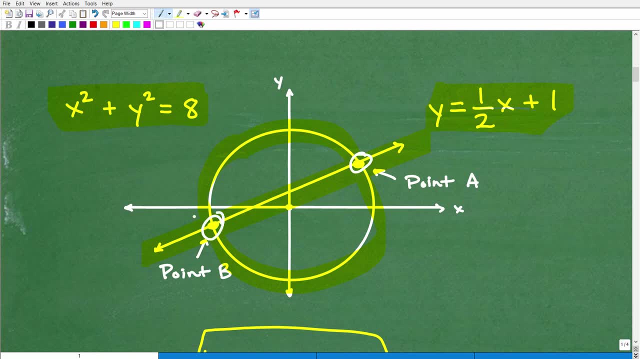 All right. So we're looking for these two points of intersection. What can we do? Well, here's the thing: You want to be thinking about, those skills that you learned in Algebra 1 or pre-algebra. And I'm going to give you a hint. 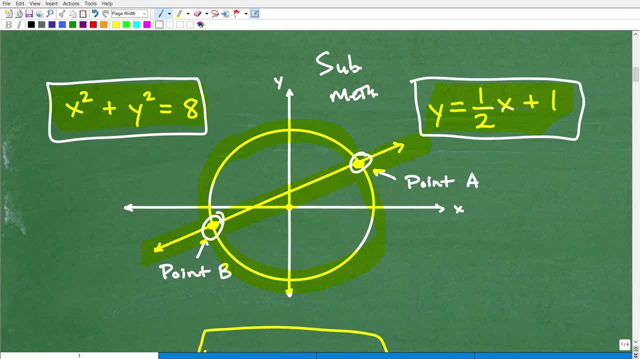 Try to use the substitution method. OK, here I have two variables, X and Y, and I have X and Y over here And this Y is already set up for me. I have Y is equal to this, So how about we substitute this Y for all of this? 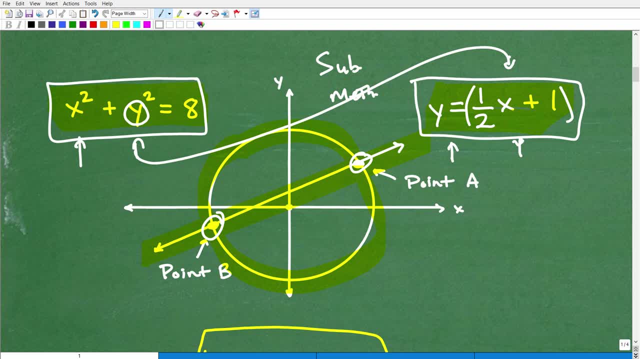 This is just going to be all of this, All of this, All of this stuff right there. OK, that is kind of the path you want to take Now. if you didn't see that, if you're like: oh, I was confused about how to solve this problem. 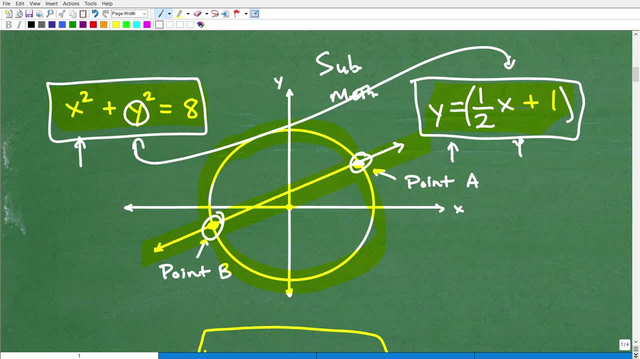 you're like, oh, this makes sense. You should probably pause this video and work out the rest of this problem, See if you can handle the algebra that goes along with this. But what are we looking for? OK, well, we're looking for as our solution: 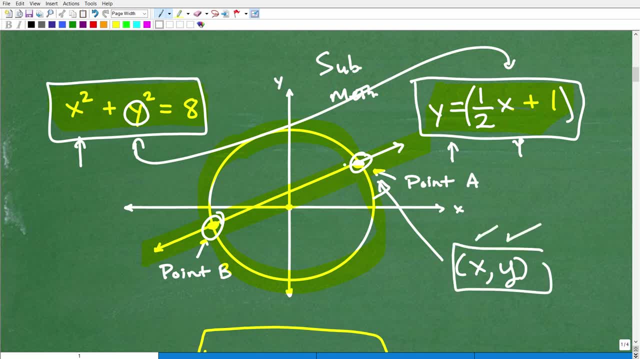 We're looking for an X and a Y x and one y that represents this point, And we're looking for another x and another y that represents this point. Now, are these x and y values going to be the same? No, it's impossible for them to be the same, because this location is not this location, right? So? 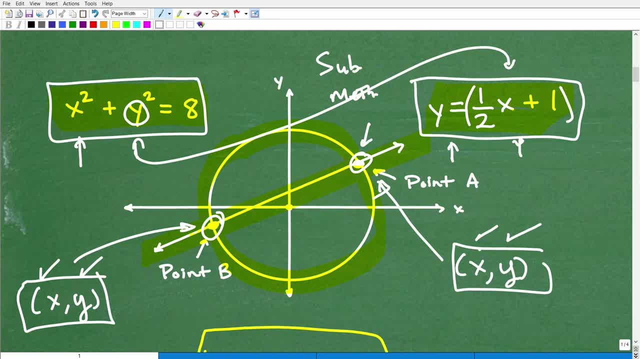 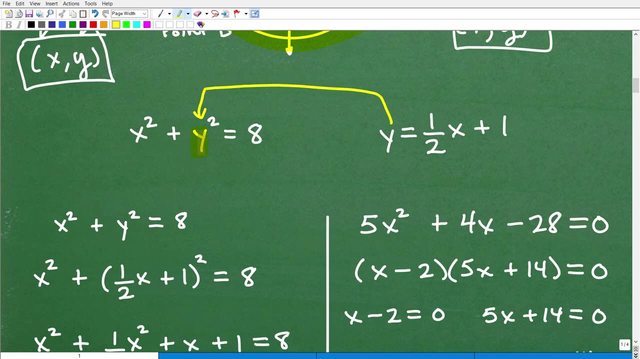 we're looking for two different x values and two different y values. So hopefully now you kind of see the big picture. Now let's get into the algebra, All right, So again, what we want to do is use the substitution method. We're going to replace that y, okay, because we know y is. 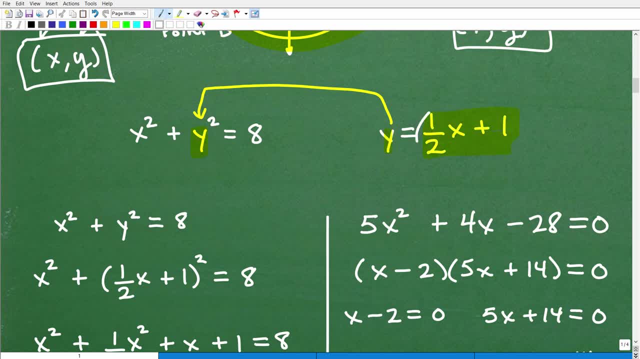 equal to all of this. We're going to replace this y with this And anytime you're using the substitution method, you want to use parentheses. So let's go and focus our attention over to the left-hand side here and plug in this right here: one half x plus y. 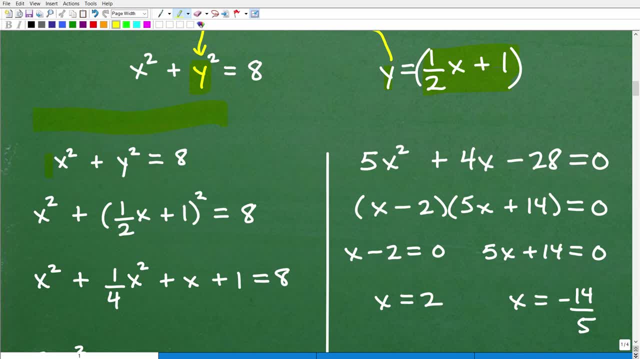 We're going to replace this y with one half x plus one. So here is our equation for our circle. Now I kind of wrote a little bit smaller here so we can kind of see what's going on, but hopefully you can kind of follow what I'm saying. Okay, So I want to replace that y. 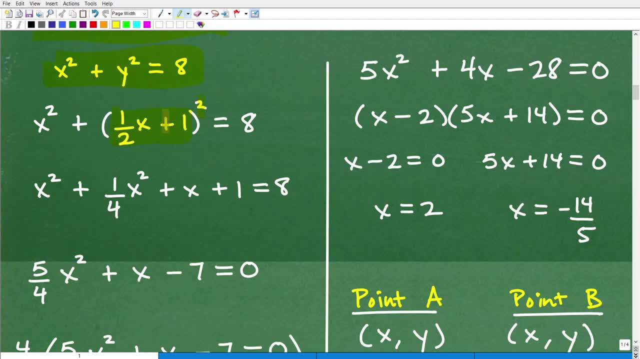 with one half x plus one and we're going to square it because this is y squared. But now I have one equation with one variable. That's what the substitution allows us. It's all in x. I'm sorry, this equation here is all in that one variable, x. So I have 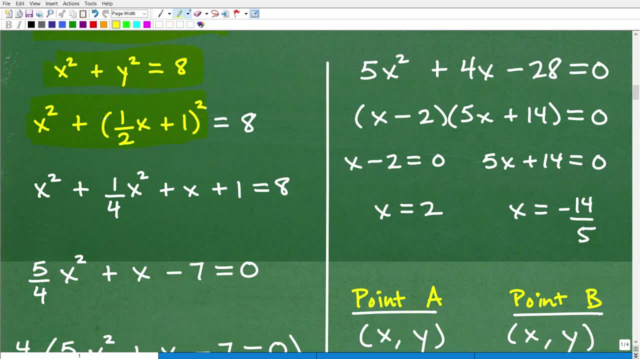 x squared, plus all of this. And now this really comes down to your ability, to you know your algebra skills and your ability to do things in algebra like multiplying square and solve quadratic equations, et cetera. All right, So here we go: X squared, one half x plus one squared I. 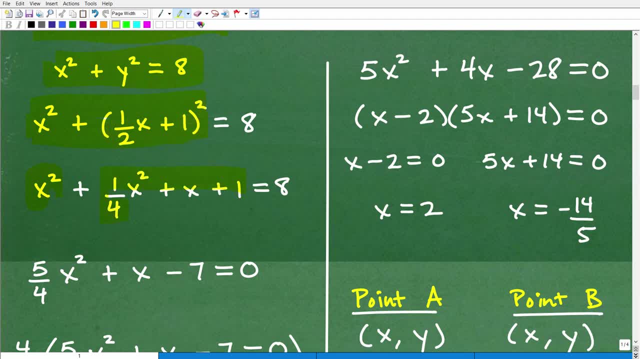 multiply this by itself. I can use the foil technique. You should get this. If you don't know how to do any of these subskills, I'm going to tell you right now. you need to thoroughly review a lot of different things in like the algebra, one level. 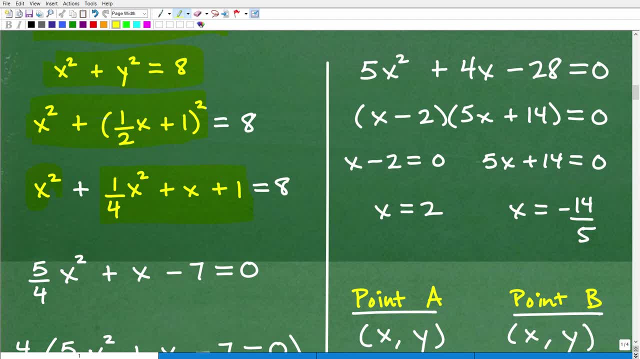 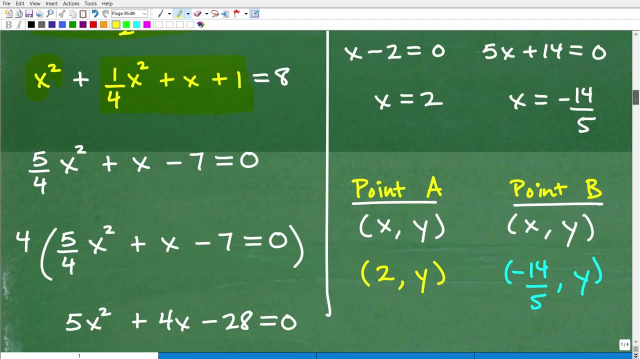 So I would probably direct you towards my algebra one course, Okay, So check that out, That will help you tremendously. I do have additional videos on all of these little topics as well. All right, So let's continue to work this problem out. So here I have x squared plus one fourth x. 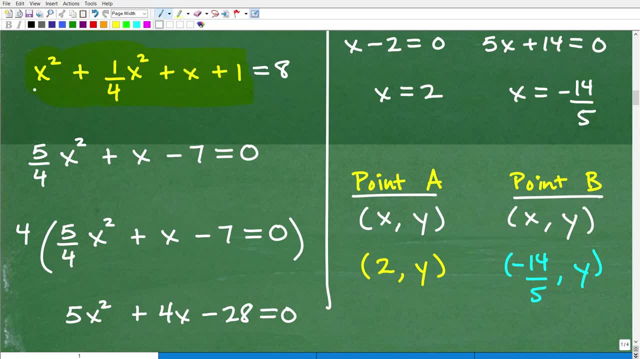 squared plus x plus one, So I can add one x squared plus one fourth x squared, And of course all of you are experts at fractions. This is the same thing as four over four. So all the x squared and x squared are four over four, or one x squared plus one. fourth x squared. 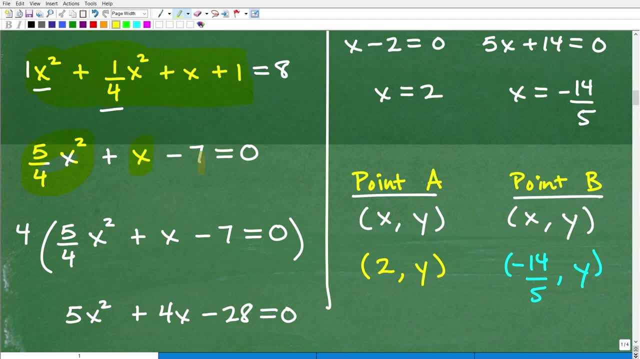 gives me five fourths x squared plus x minus seven. Now what I did here is I subtracted eight from both sides of the equation And I'm writing this thing, or I want to write this thing in standard form: Okay, And it's pretty much highest to lowest power, And you set this thing equal to zero. 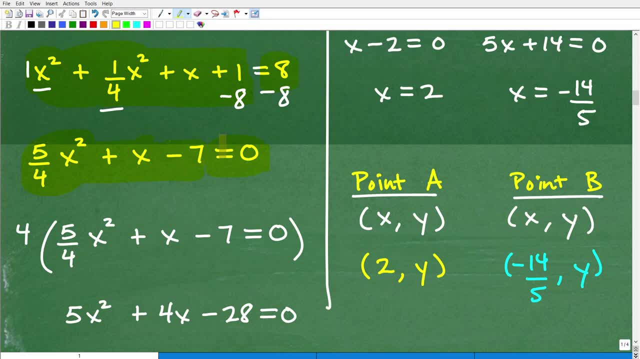 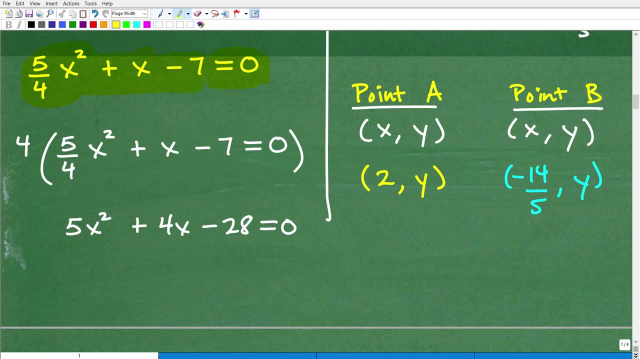 because what are we dealing with here? We're dealing with a quadratic equation, All right. So I'm going to clear away this fraction, this leading coefficient here, And that's just a fancy term for the coefficient or the number in front of the x squared. So let's get rid of that. I can. 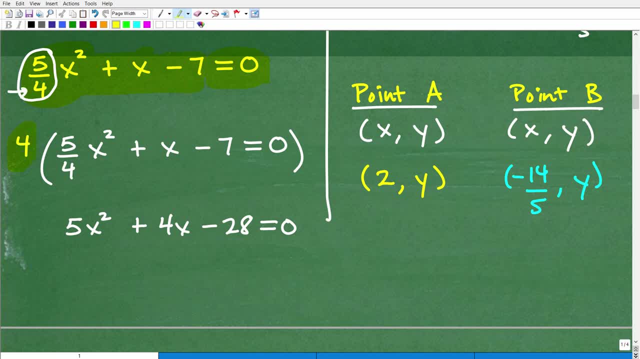 always get rid of all the fractions by multiplying by the LCD. LCD here is four, So we're going to multiply the entire equation by four. Now, if you didn't want to do this, that's perfectly fine. You could solve this quadratic equation using this coefficient, But you know that would be like. 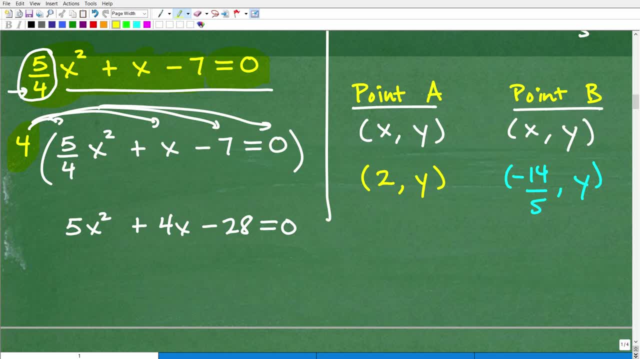 more work, Then is necessary Always clear fractions, if you can. So when I multiply four by five fourths, you're going to get five x squared. Four times x gives me four x. Four times this negative seven gives me negative twenty eight, And four times zero is zero. Okay, So here is our quadratic. 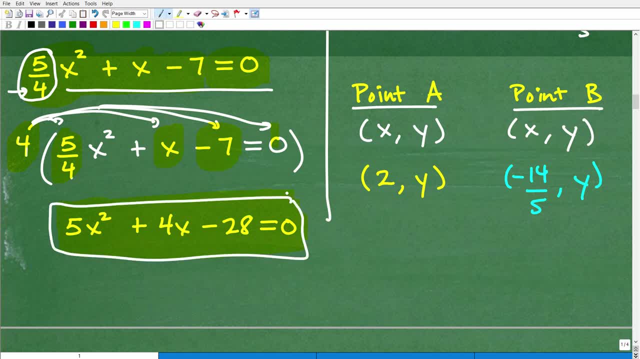 equation And we still don't have the solutions for this. But what do we know? When I solve for x, quadratic equations always have two solutions. Okay, So I'm going to have two solutions. I have one solution for x and another solution for x. Two solutions, And remember, keep the big. 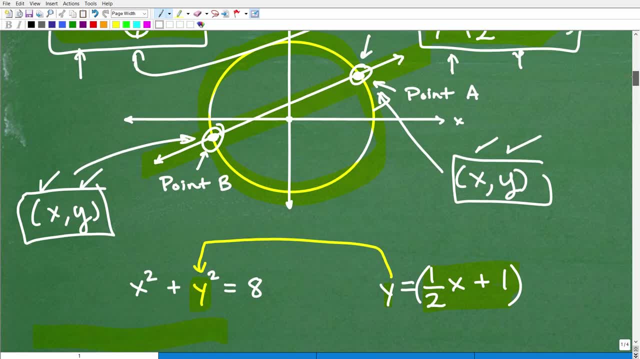 picture in mind. We're looking for two x values, right, We're looking for one x here and one x here, And because we're solving this quadratic equation, we're going to get two unique x values. That's going to represent these coordinates for these respective points. So this is making sense. Well, 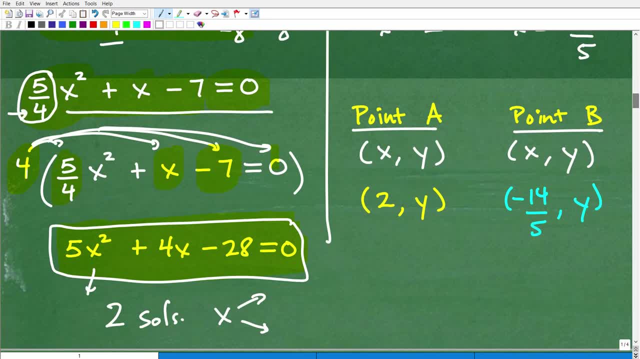 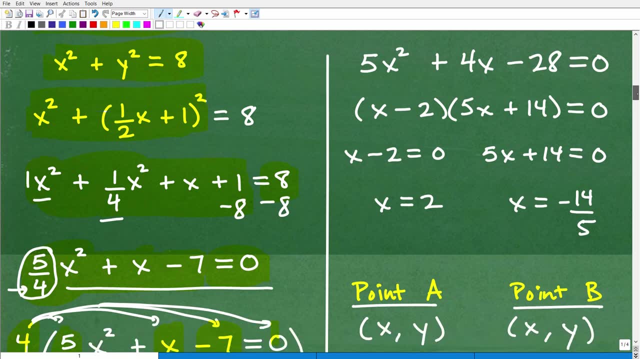 at least hopefully, it's making sense, But let's go ahead and continue on, All right, So let's go ahead and solve five x squared plus four x minus twenty eight, And we'll pick up the problem right here. Okay, So anytime you are solving any quadratic equation, 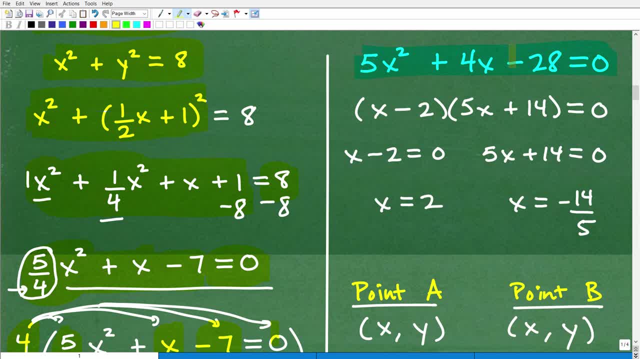 and you have a trinomial. always try to factor. That's the easiest thing to do. So this is factorable. Now, how this is factored into this, that is a skill. Okay, You have to be excellent at factoring. If you don't know how I went from here to here, you don't know how I went. 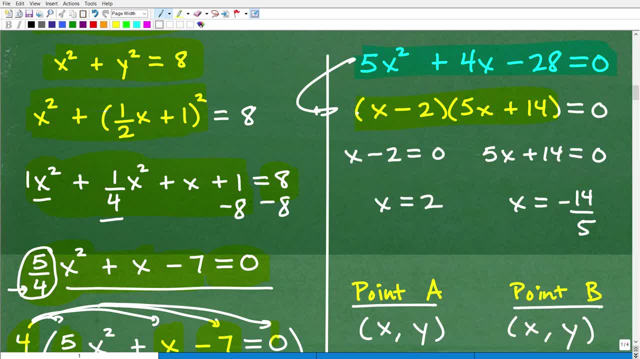 from here to here, You need to review factoring. All right, I would say probably one of the most important skills in pre-algebra- algebra one, algebra two, all of algebra- is your ability to factor. Okay, So, anyways, you want to be able to factor and we can factor. So we have this. 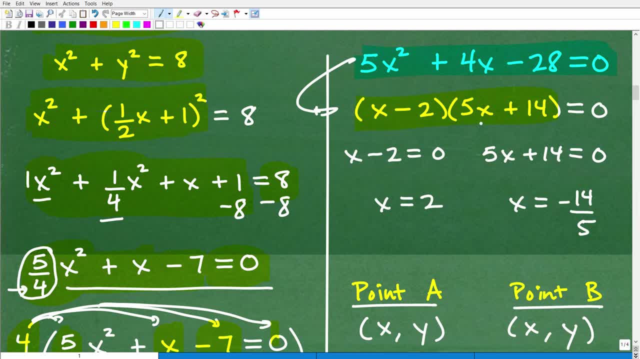 trinomial equal to x minus two times five. x plus fourteen is equal to zero. So now we can set each of these factors equal to zero. Okay, This is what we call the zero. So we can set each of these factors equal to zero product property. And when I solve these respective equations, you get: x is equal to. 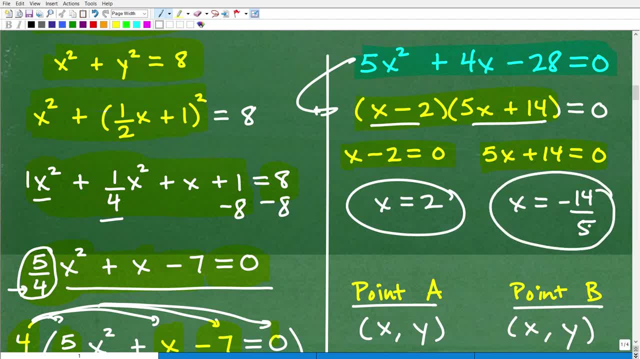 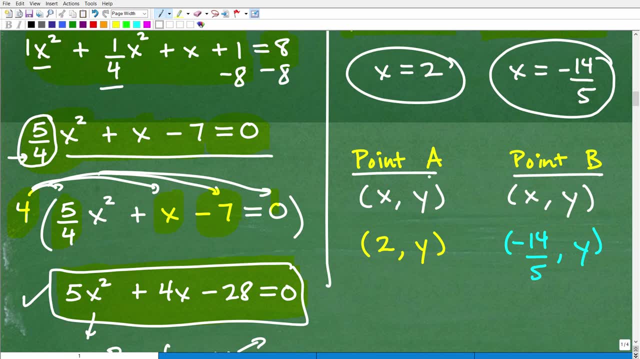 two and x is equal to negative. fourteen over five, Okay. So what does that mean, though? Well, we just found the x coordinates for these respective points. We got point A and point B, and point A, its x coordinate is going to be two, Okay. And point B, its x coordinate is going to be: 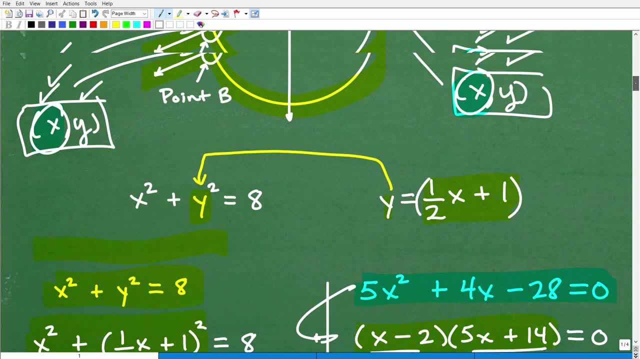 negative fourteen over five. Now, how do we know that? Well, I'm calling. how do we know which one's A, which one's B? Well, just look here. We know that point A is in the first quadrant, Okay So. 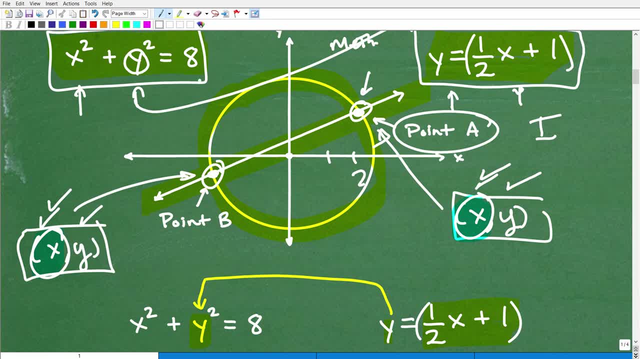 it's like one, two over here. So this point, just visually speaking, its x value, is going to be negative, right? So this is negative and it's going to be negative. So we're going to have this in the third quadrant and this point will be in the first quadrant, right, This is going. 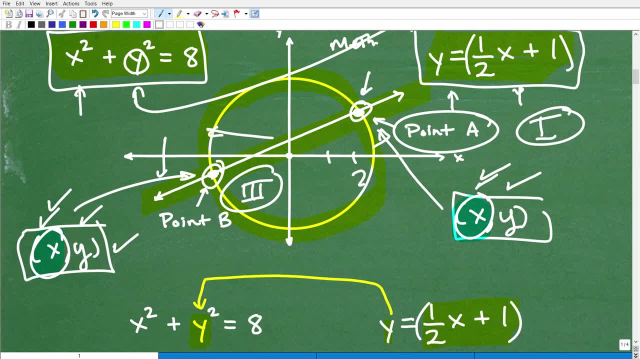 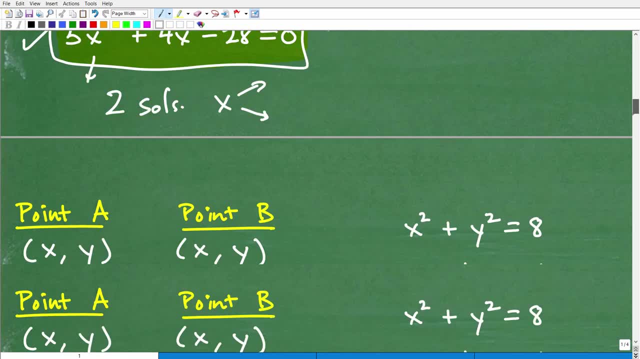 to be negative, and negative in terms of our x and y and our point B. So we're going to have point A here should be positive and positive. Okay, So we have our x's, Let's go get our y values now. So we'll pick up the problem right here. So how do we get y when we have solved for? 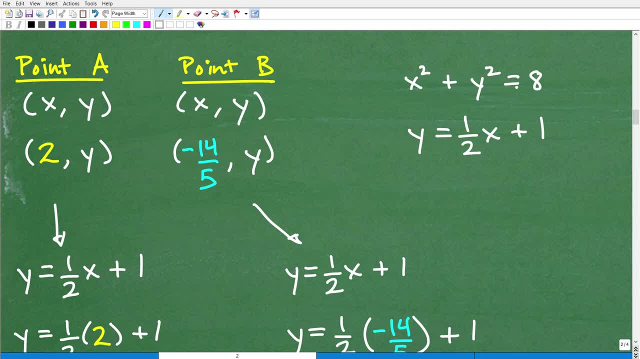 x. Well, we have two equations that involve both x and y, So I can either use this equation or this equation. Which one's easier to use? Well, obviously this is the easier equation to work with, because we are solving for y, and this is super easy. for solving for y, We have x, We just 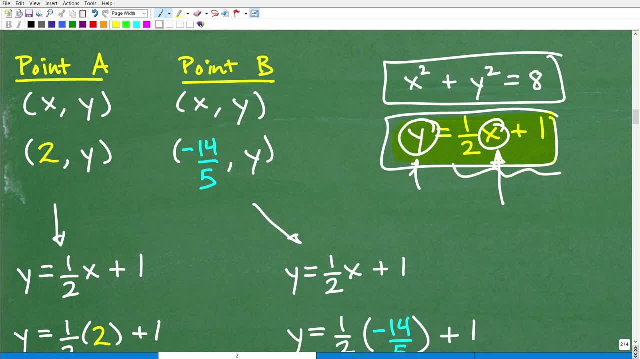 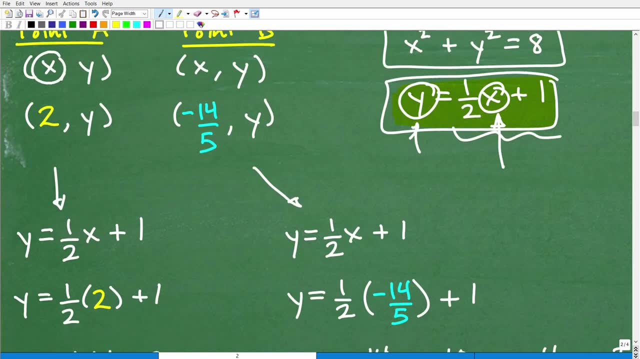 plug in our x values here, do this number crunching and we will get y. And let's go ahead and do that right now for these respective points. Okay, But look here we have to do it twice, because we've got to plug in x when x is two to get the y value for that point, And then once. 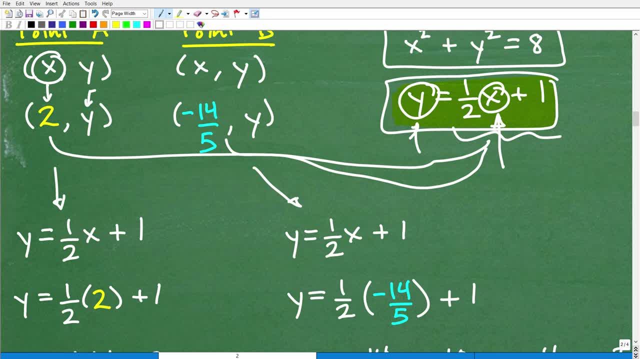 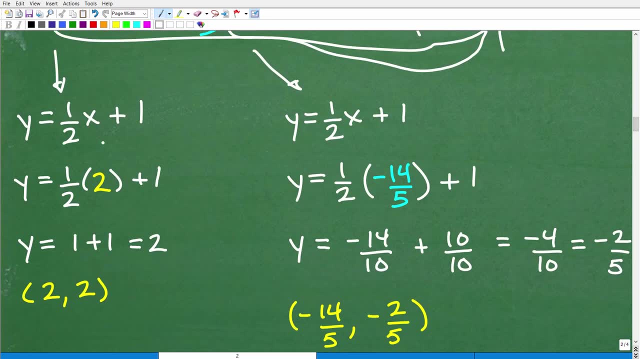 we're done doing that. we've got to plug in this x value into the same equation to get y for the other point. Okay, So let's go ahead and do that now, And you can see I already did the work here. when x is two, y will be two. You can see the work. So that point is two: two. And when x is, 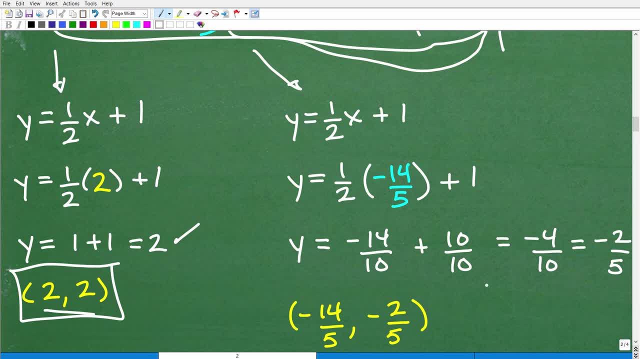 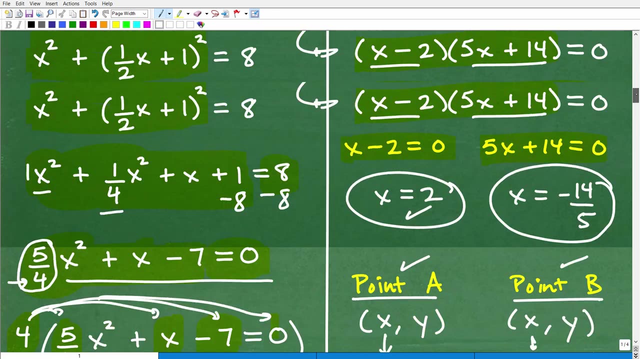 negative 14 over five. y is equal to negative two fifths. Of course you can see all the work there just to kind of double check this stuff. And that is that second coordinate. Okay, So this is how you get these two points, And this would be the solution to this non-linear system. Now, does this? 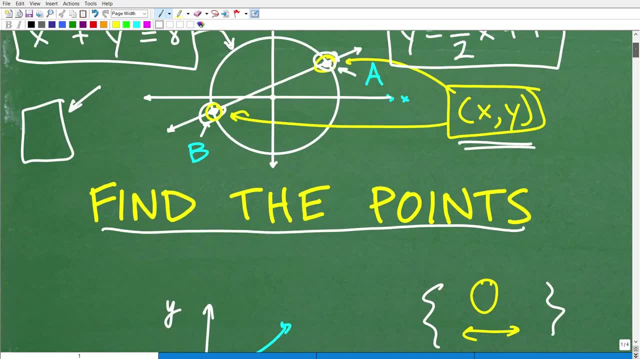 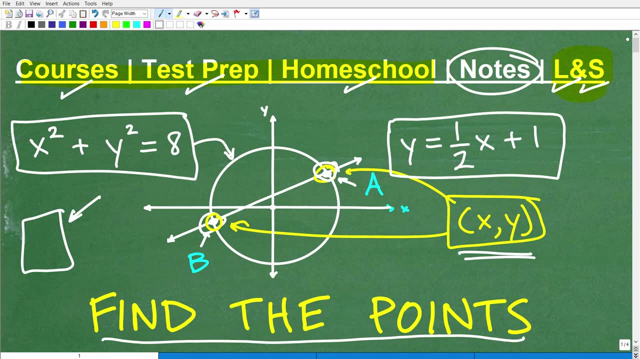 seem like a lot of work. Well, yes, it is a decent amount of work. I'm not going to try to lie to you and say, hey, this is an easy problem to do. It takes one, two, three. No, at this level of math, you know, and this I would say is a kind of medium level. 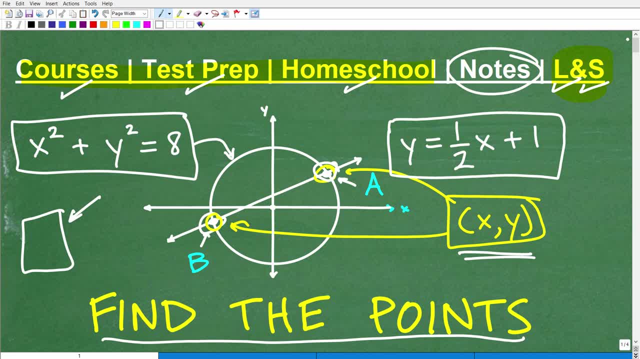 problem: Okay. When you get into more advanced mathematics, some problems will take you multiple pages to do, Okay. So don't feel like man. maybe you're off track because you're doing a lot of work. You're doing a lot of writing. You're like boy, this problem is going forever. Yes, At this. 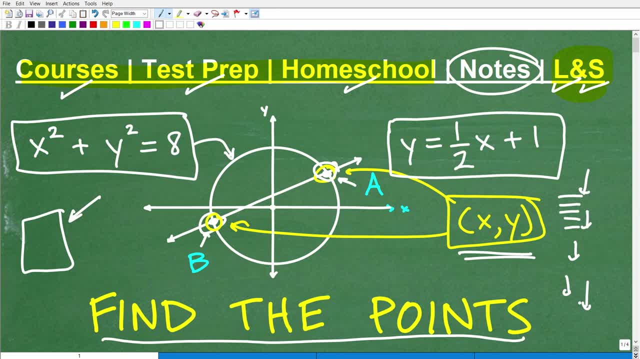 level of math. sometimes these problems do take you a little bit longer, But if you're doing a lot of, you know space. that's why you never want to be too restrictive in terms of like the paper you use. Get yourself plenty of paper, Be nice and neat, Use pencil and take whatever room. 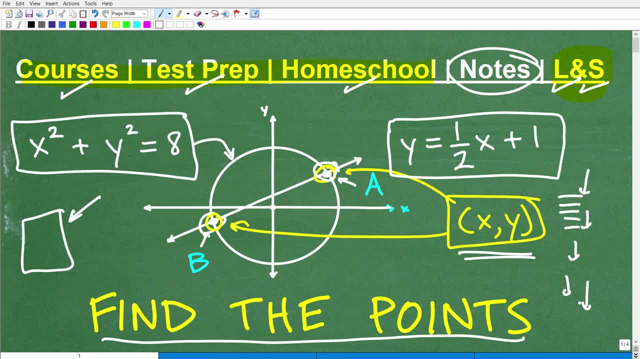 you need to keep writing out these steps. Don't shortcut writing things down because you're trying to save space on your paper. That's definitely a big no-no, And once you're done you should go back and look at your work And can you read the solution? Can you kind of like?